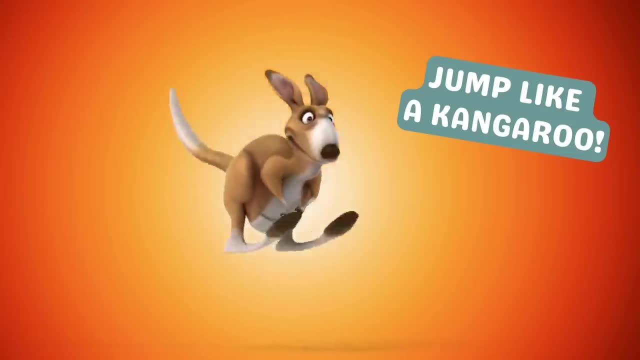 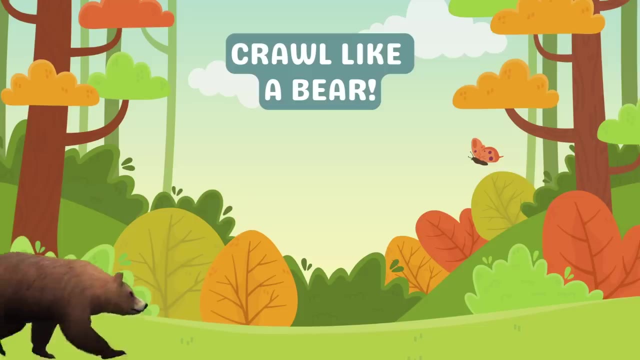 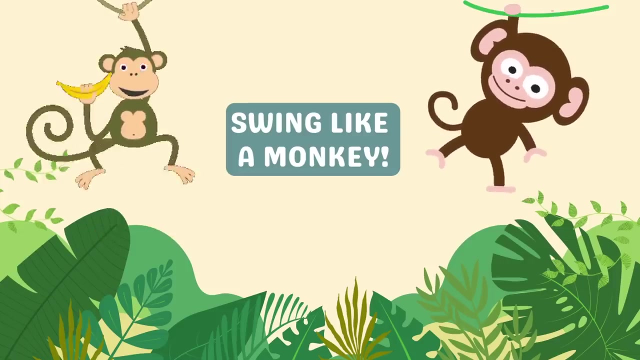 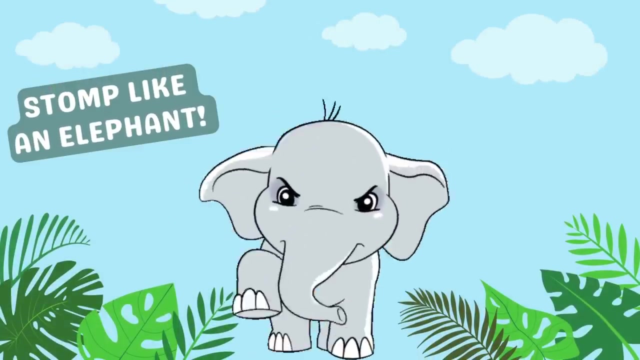 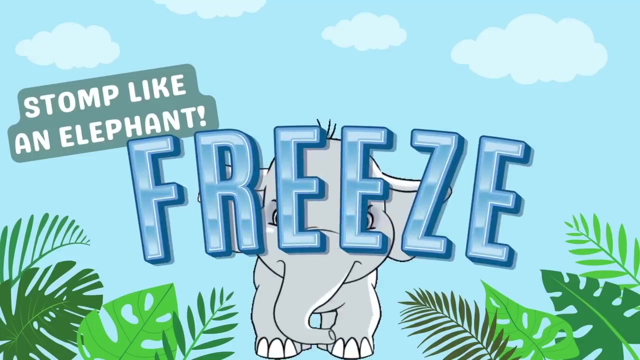 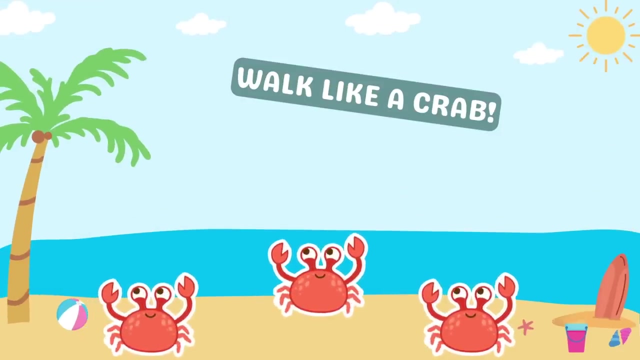 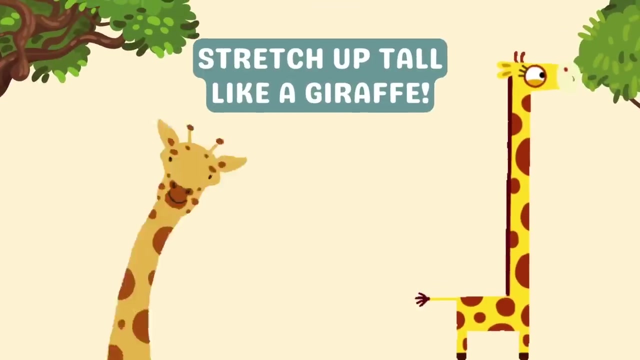 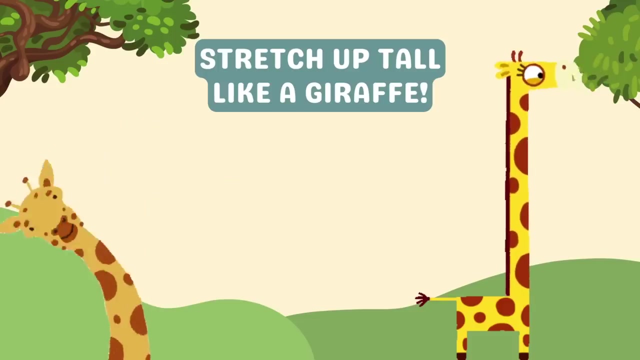 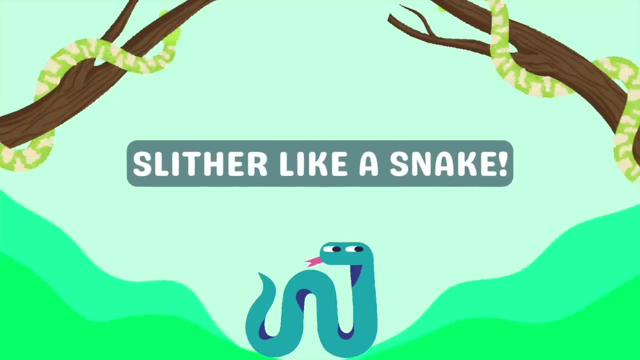 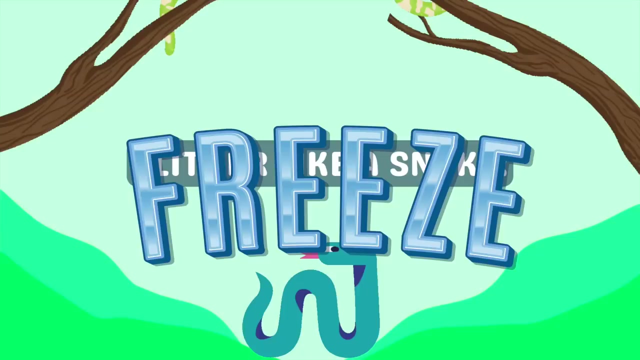 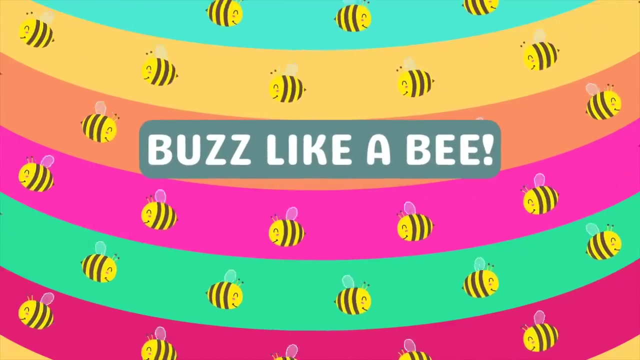 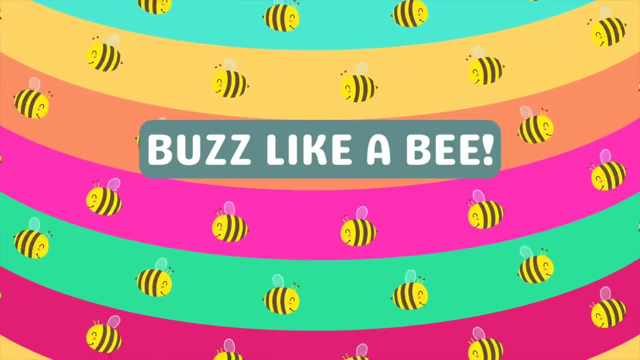 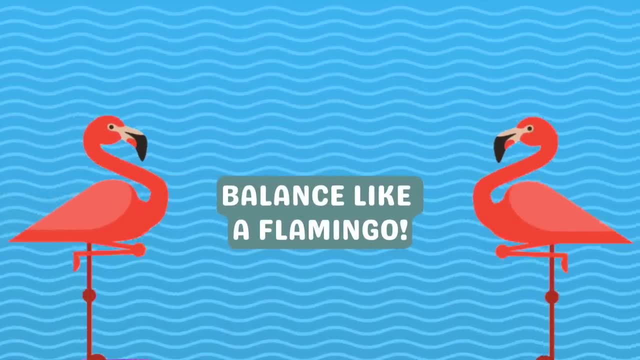 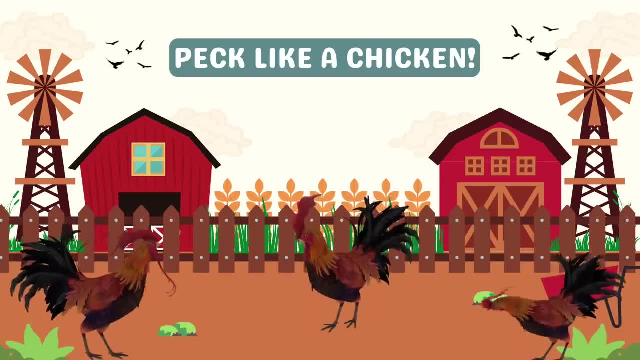 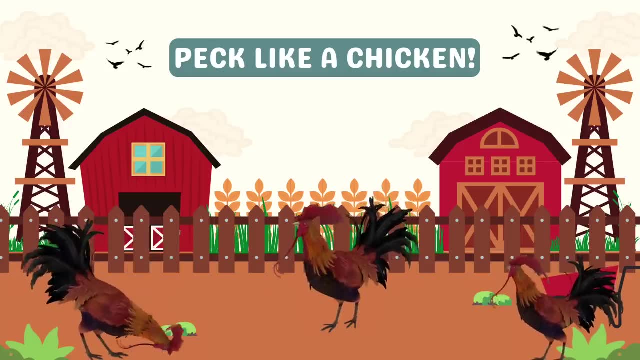 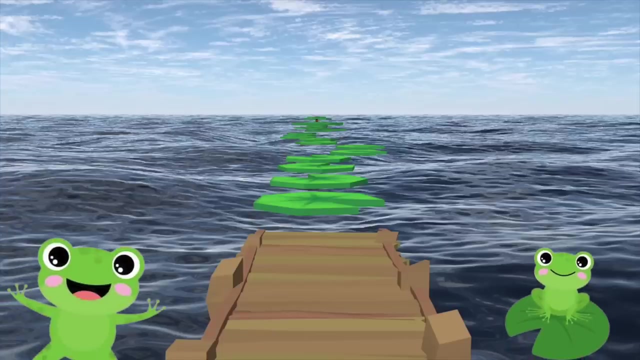 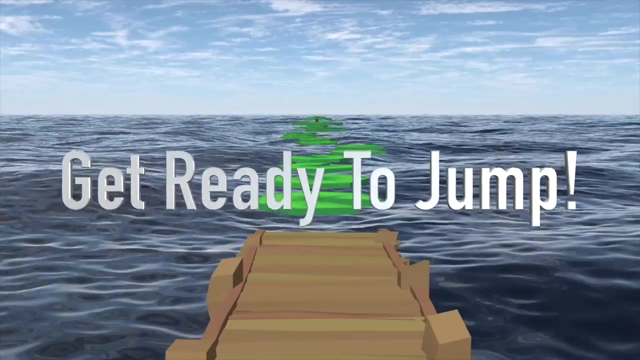 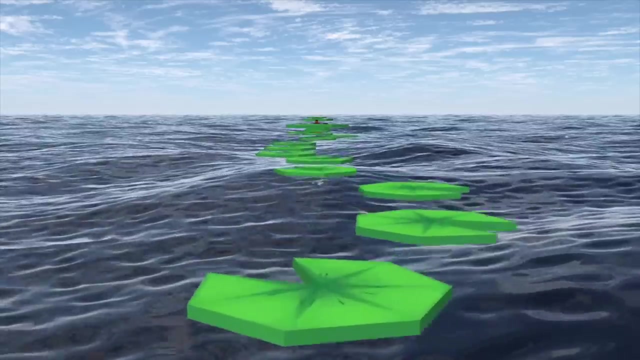 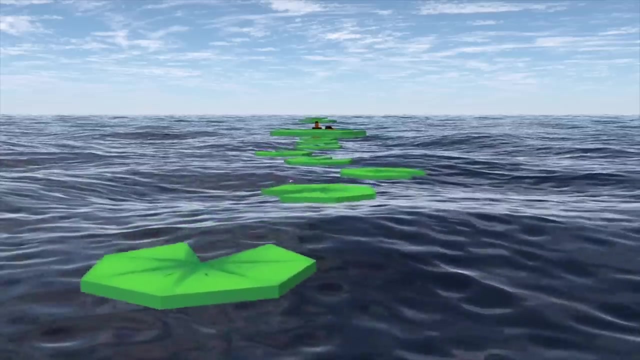 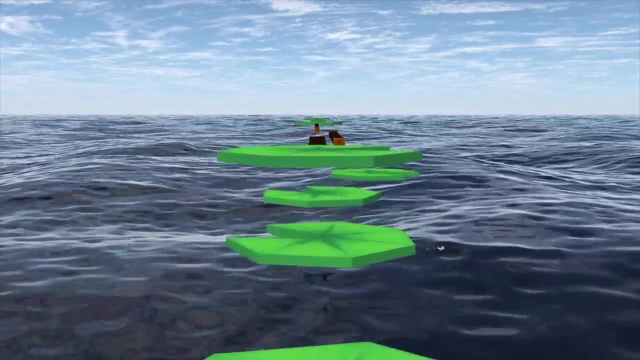 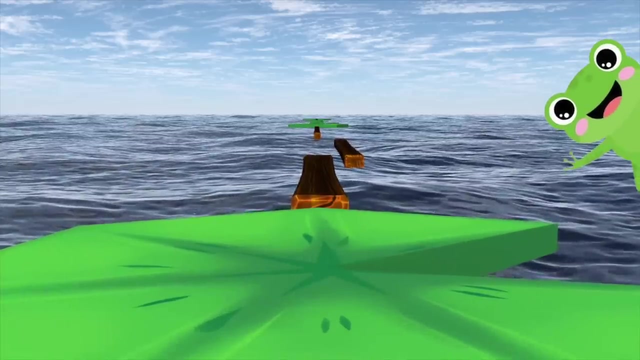 Peck like a chicken. Hi friends and welcome to lily pad lead. The rules are simple: Jump on the lily pads and don't fall in the water. Are you ready? Let's go, Let's go, Let's go. 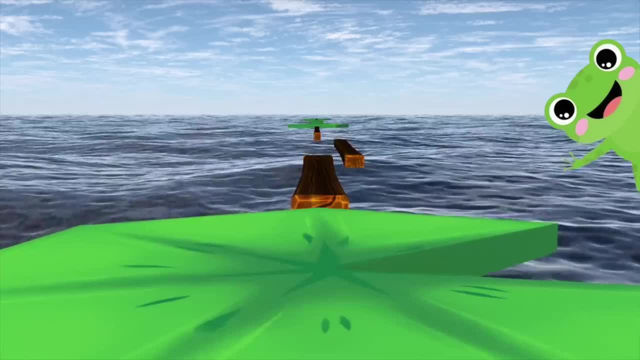 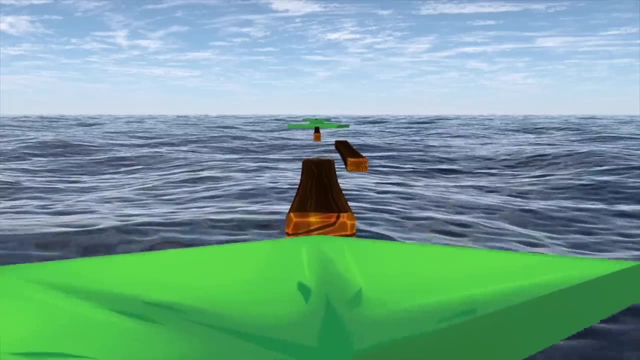 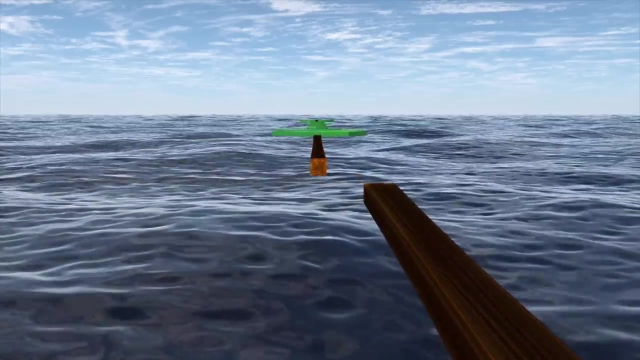 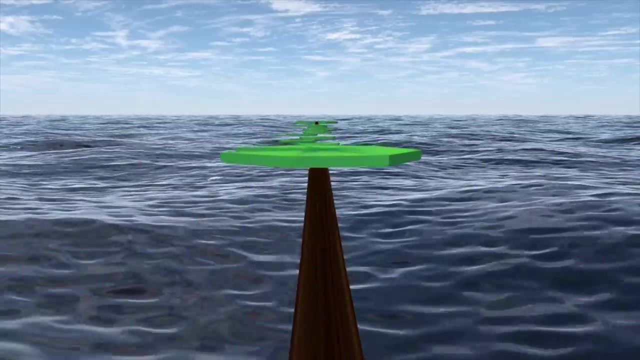 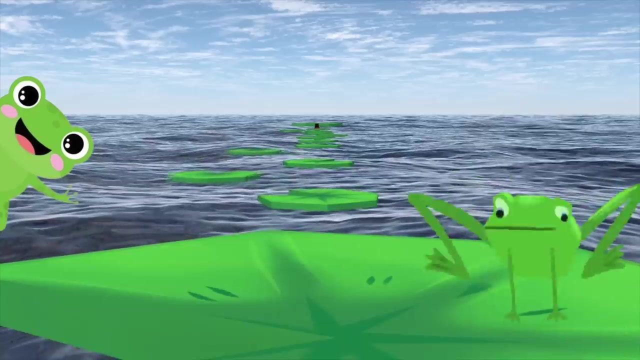 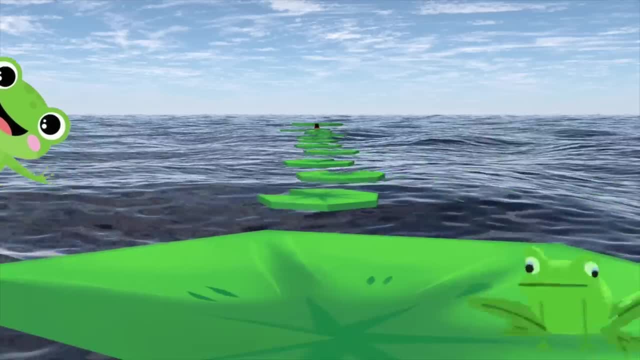 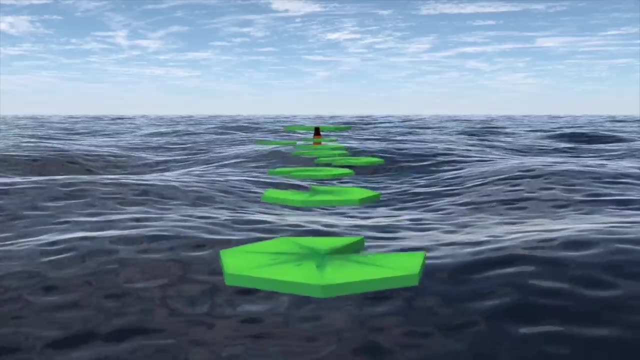 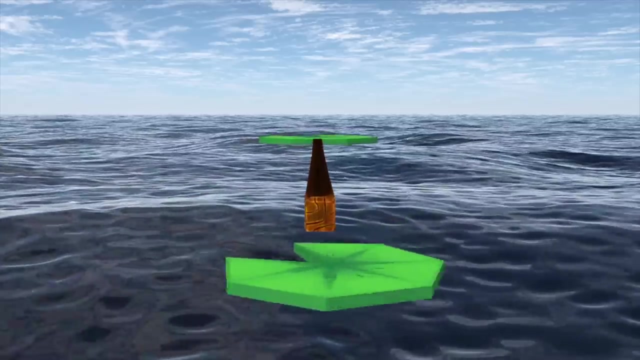 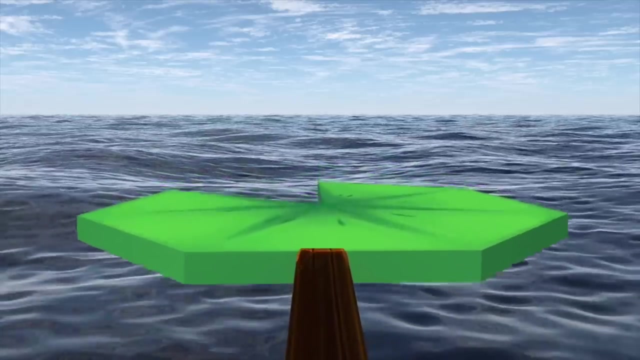 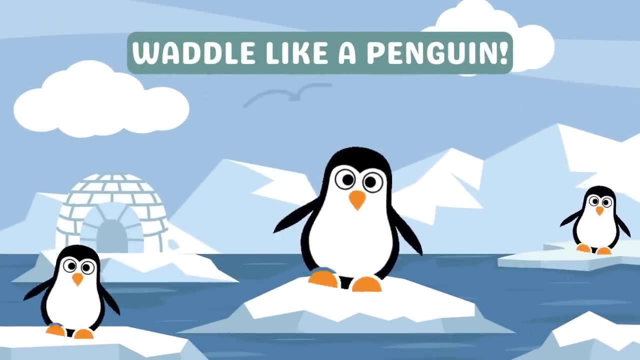 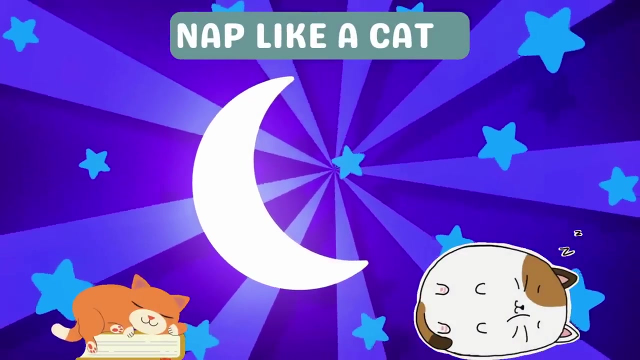 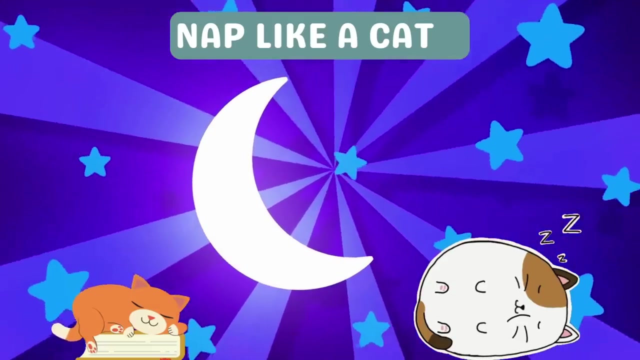 It's the final round. Let's see what you got. I knew you could do it. Now let's get back to the dance party. Waddle like a penguin, Nap like a cat, Swim like a fish. Swim like a fish.